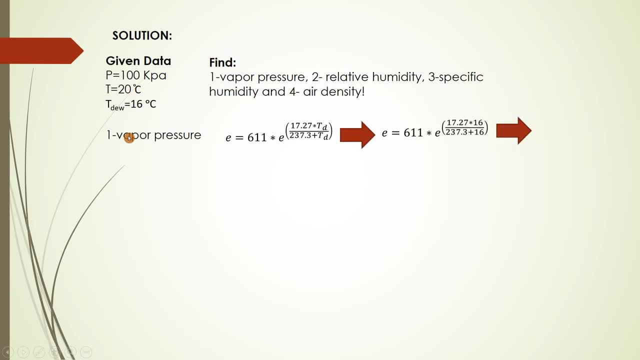 So vital pressure equals to 1818.82 pascal. That is the solution for the first one. The second one is relative humidity. Equation for relative humidity is RH, equal to vapor pressure divided by saturated vapor pressure. We don't have value of saturated vapor pressure, so we have to find it. 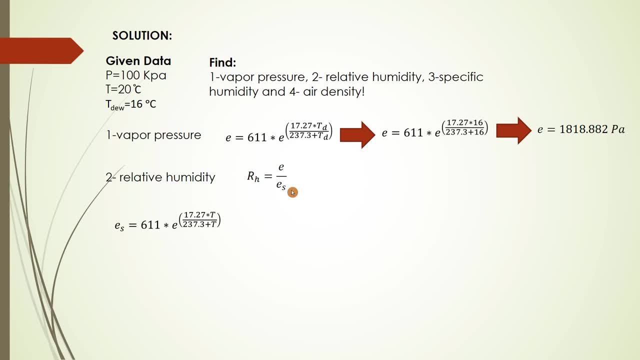 That is the equation for saturated vapor pressure. It is the same as a vapor pressure, But we use air temperature instead of dew temperature. So just put air temperature in the equation, You can find the saturated vapor pressure. So saturated vapor pressure equal to 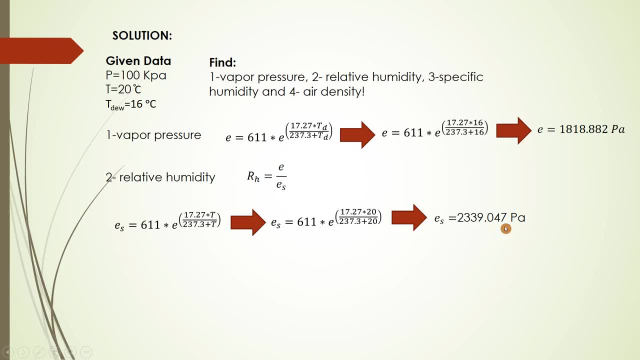 2339.047 pascal. Now we can find relative humidity. Just put the value of vapor pressure and saturated vapor pressure in the equation, So relative humidity equal to 78% Regarding the third one, which is specific humidity. That is the equation of specific humidity. 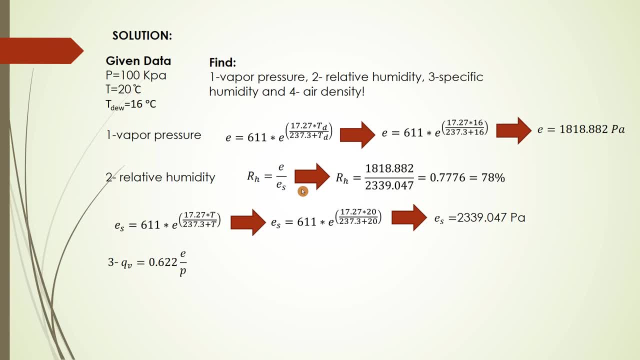 Which is equal to 0.622 vital pressure divided by air pressure. But we have to convert pressure from 100 kilopascal to pascal, So it equal 0.622 vital pressure in pascal And air pressure multiplied by 1000 to convert to pascal. 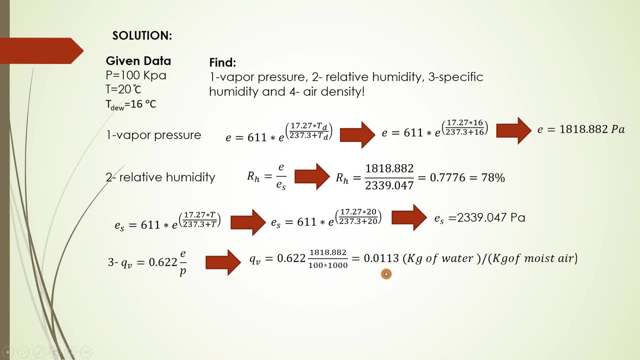 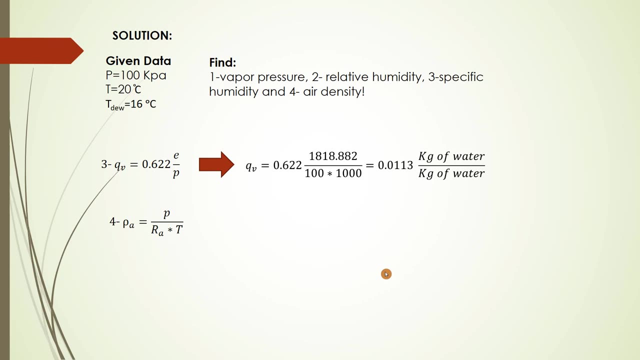 So it equal to 0.0113 kg of water per kg of moist air. That is the specific humidity And the last one is air density. That is the equation for air density, equal to pressure over RA factor multiplied by T. But we have to take care that T is in Kelvin.